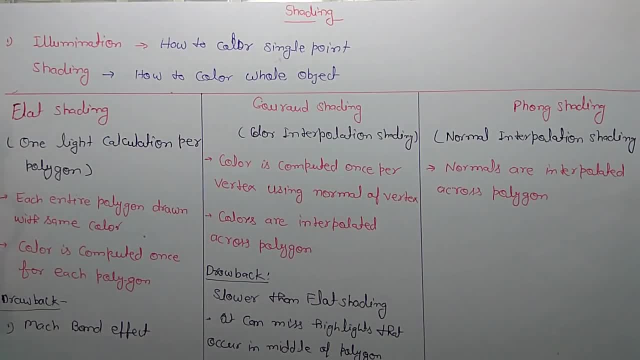 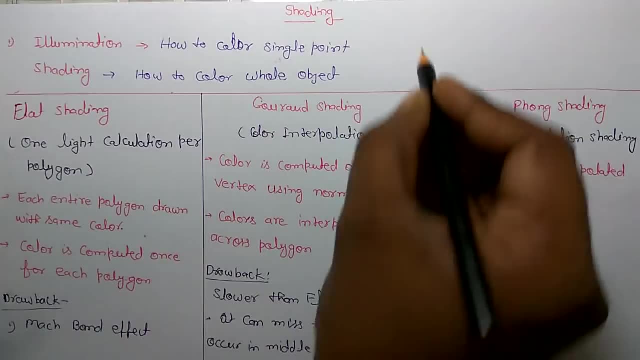 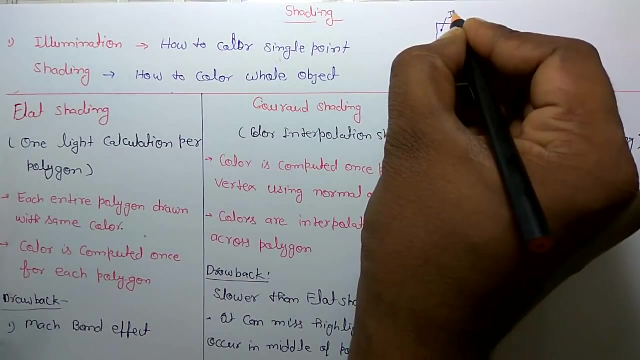 Today we are going to learn shading. In the illumination model we have found that, how to color, how to calculate the color of single point, For example, if there is an object, so we are able to find intensity at a particular pixel. Now shading, see using this intensity. 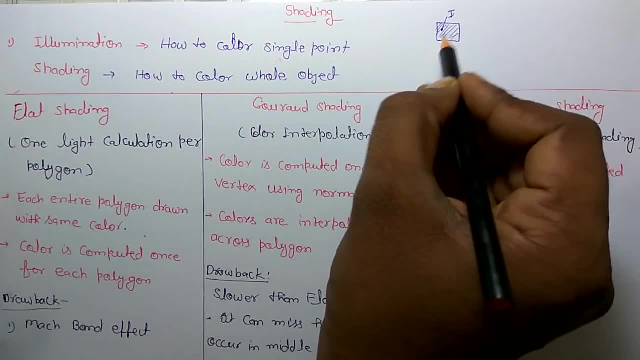 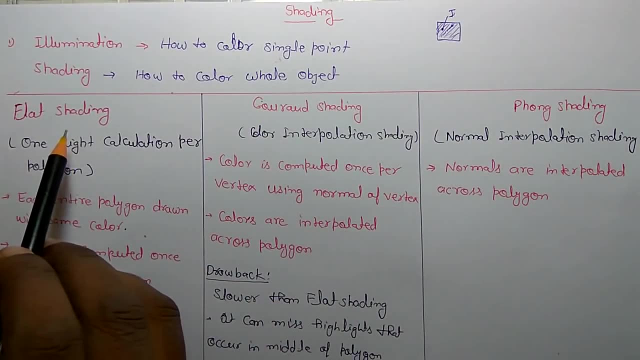 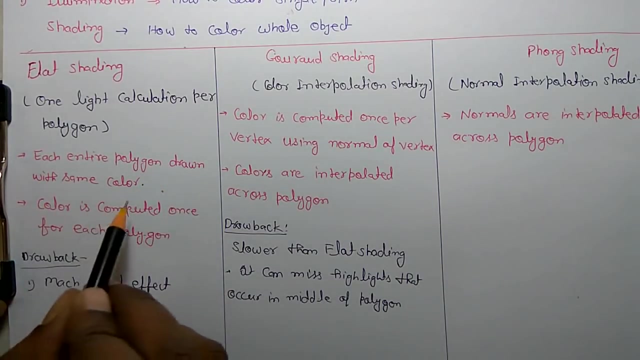 how you can color it object. So shading is related to coloring whole object. So basically there are three types of shading: flat, corad and fang shading. In the flat shading, each entire polygon drawn with same color. one light calculation per polygon, For example: 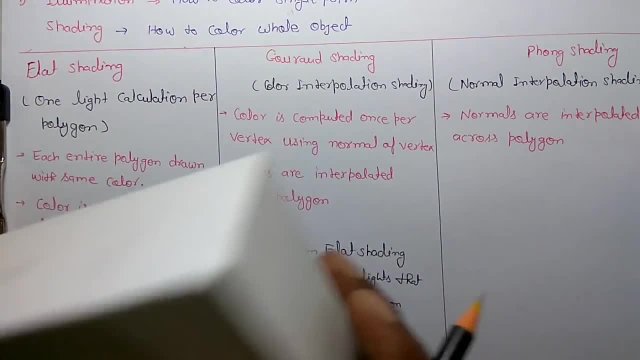 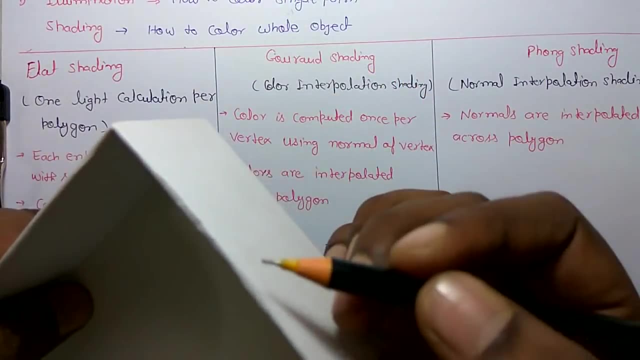 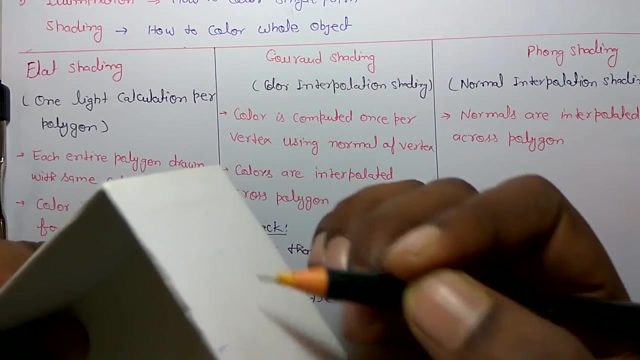 if it is a polygon and this side it is a polygon and we want to color it with some color. So, for example, if I have divided it into two parts, first I have calculated this intensity at this place and complete shading we have performed at this place and remaining I have 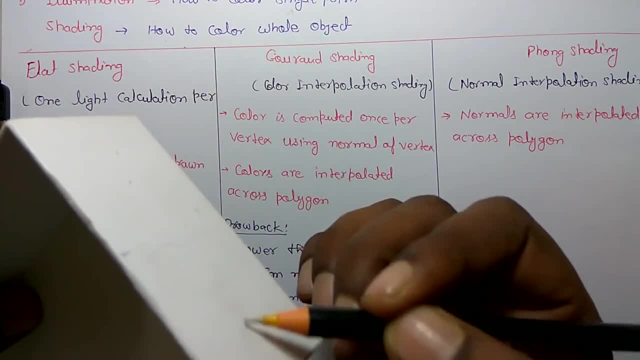 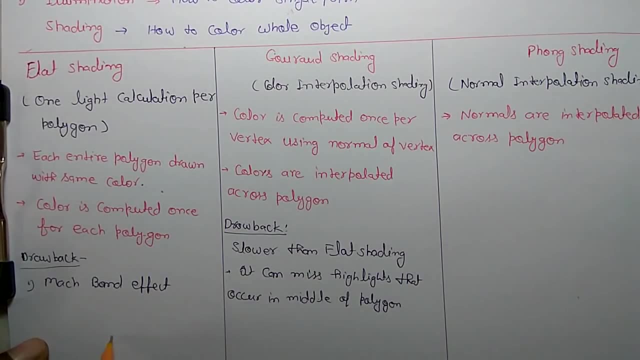 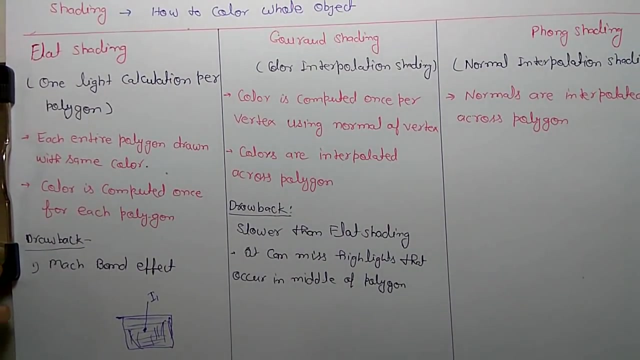 again calculated intensity remaining half polygon and color it. So this is a flat shading. In the flat shading, if there is object and you have to find intensity at one pixel, and using this intensity or this color you can color whole polygon Or shade whole polygon. So for each polygon color is computed at the once. So drawback: 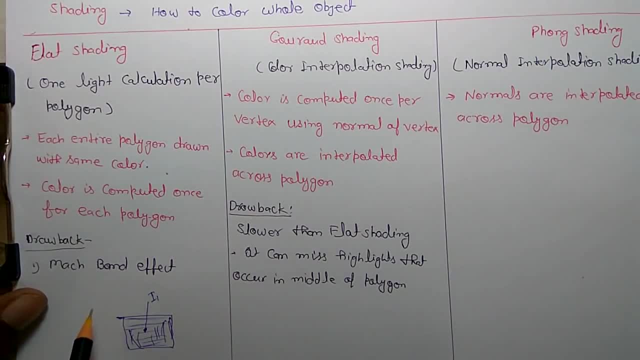 is match band effect. match band effect. what happens in case there is polygon and we have divided it into two parts, that first we have to color this, then we have to color remaining this part, whereas all of them were of same color. so i1 and i2, you have calculated and 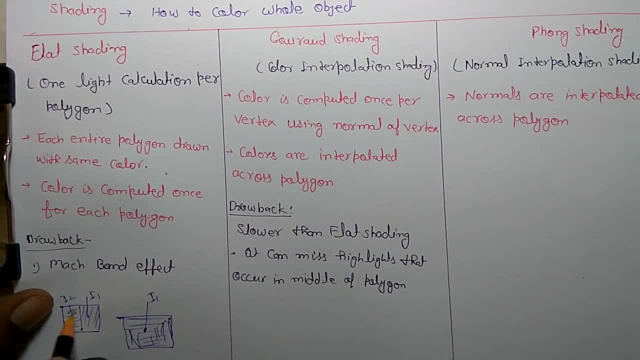 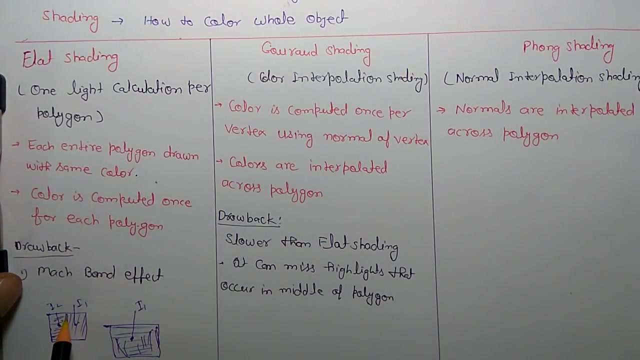 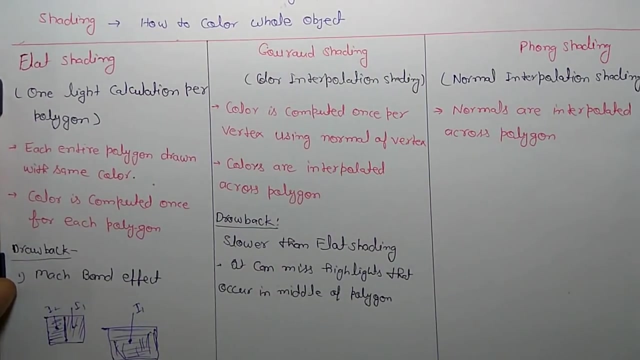 performed this color. so what will happen between these two, which we have logically divided, as we discussed before? a line appears due to intensity color change, so this is match band effect. so, for example, if we got more intensity here and a little slower here, so a color difference appears on boundary line here, so this is match band effect. 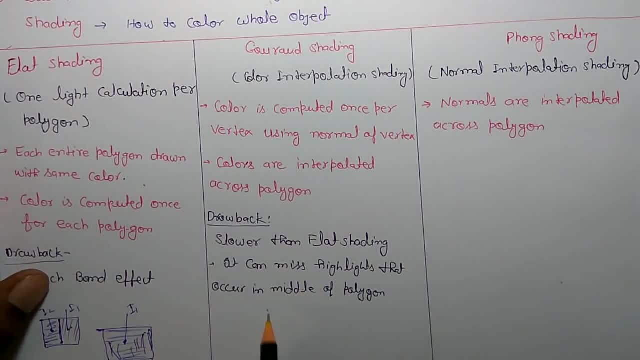 next is garage shading. what is in garage shading if there is a polygon, and it is point P1, P2 and P3.. So in grout training what will happen is that on each vertex you will find the intensity and on each vertex intensity and color. that is I1, I2 and 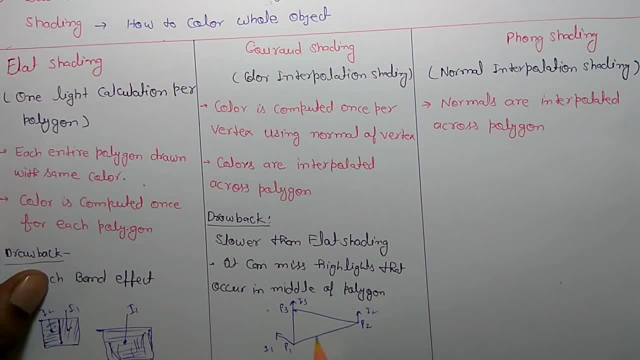 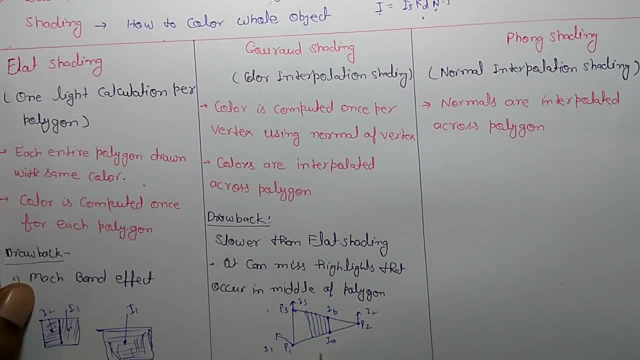 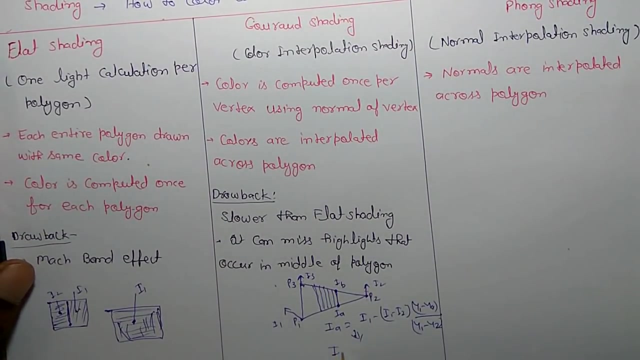 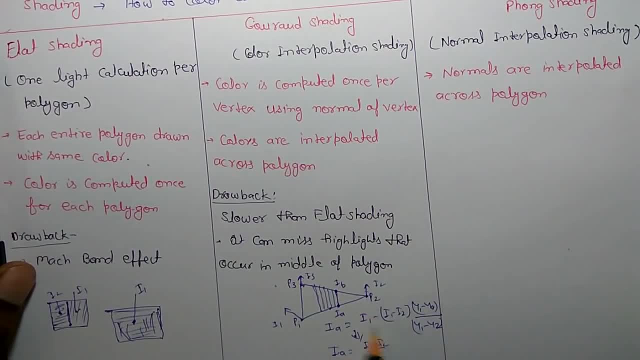 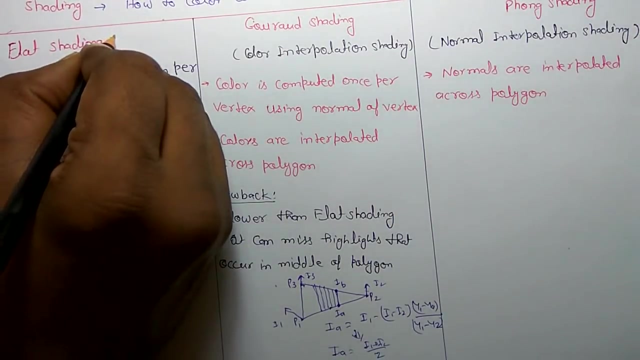 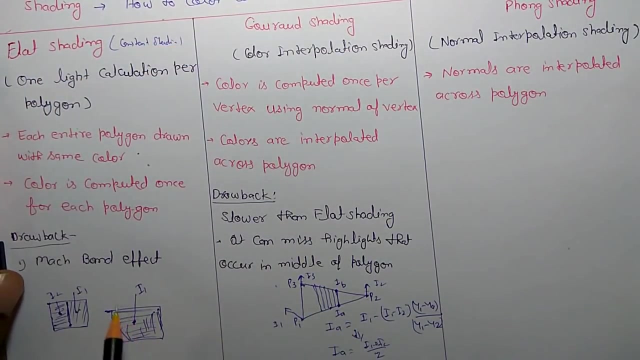 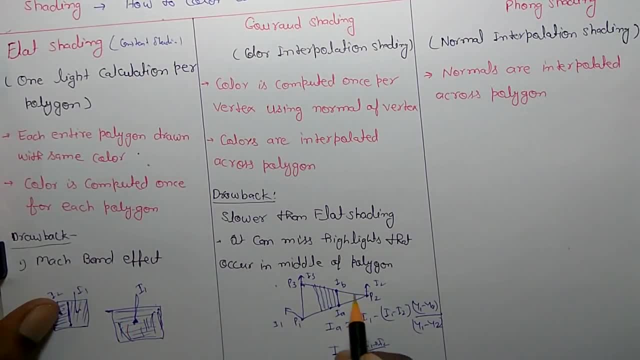 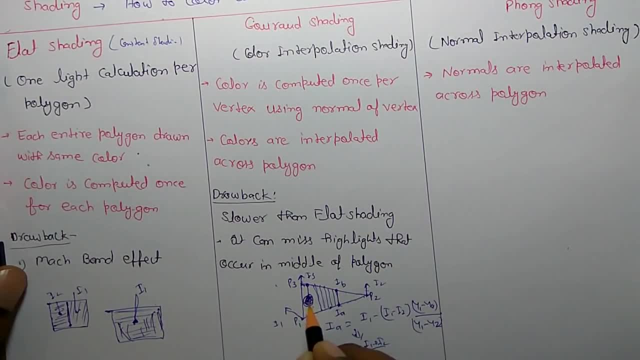 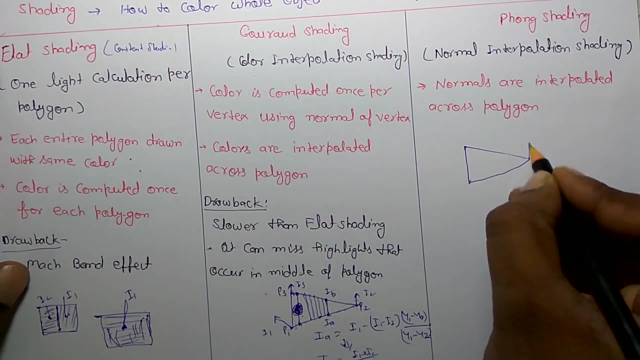 on this base you have colored. if there is any specular reflection in the middle then you can miss it in gorar shading. and this drawback you can remove from fong setting. so what does fong setting do that? any. if you have polygon, its normals first, it is calculated at vertex. 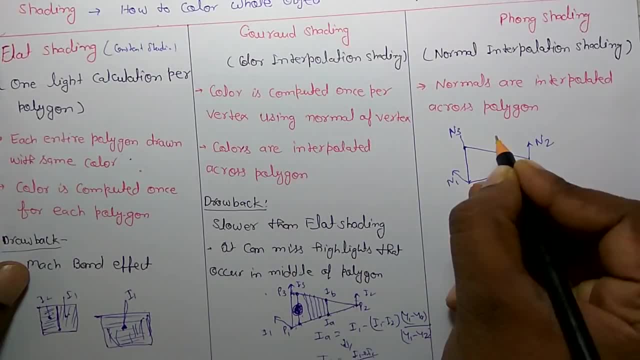 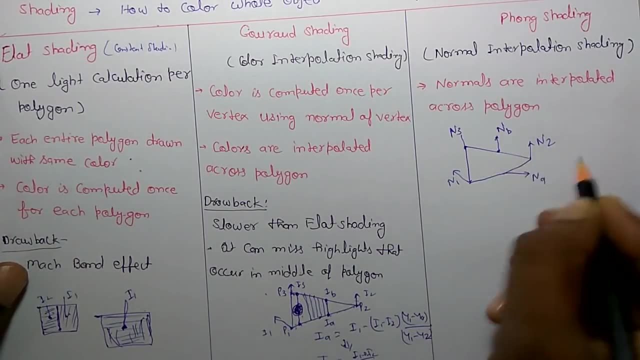 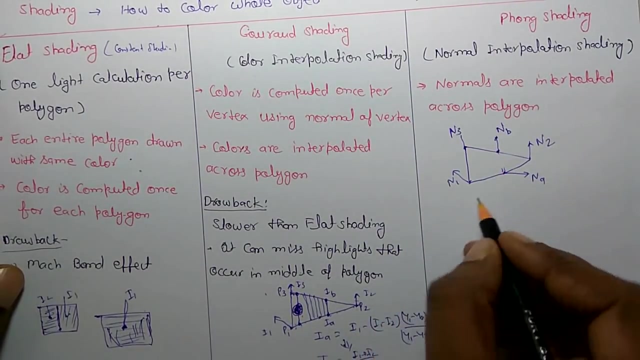 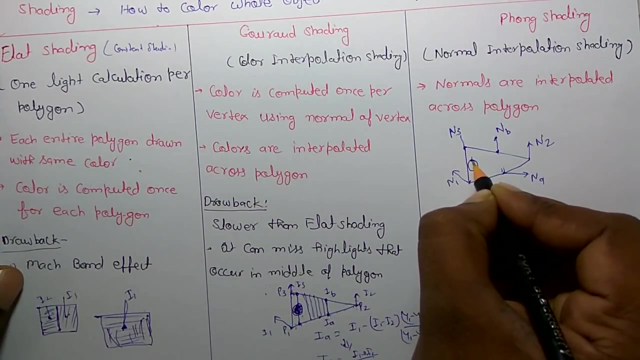 plus, at this place also, your normals will be calculated. so in this, first we calculate normals at every pixel, then we find its intensity. so what will happen in case if there is any specular part? so first we will find normals on this and then we will find color intensity. 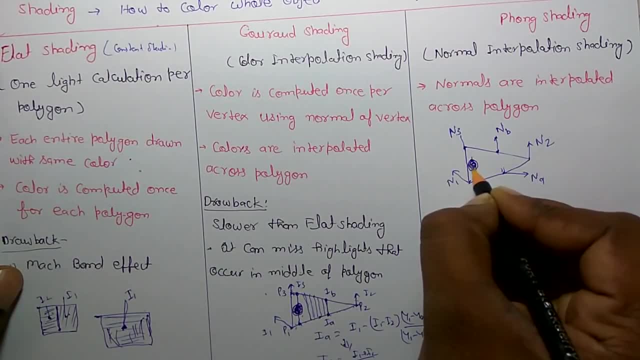 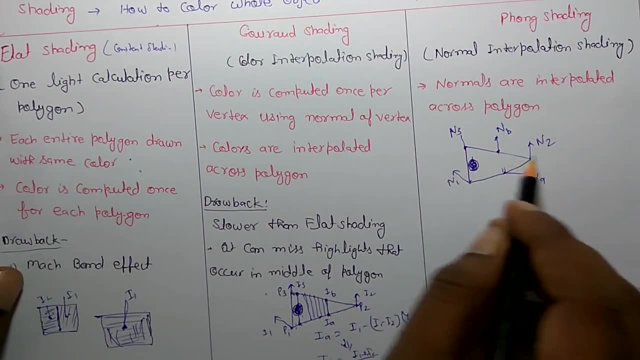 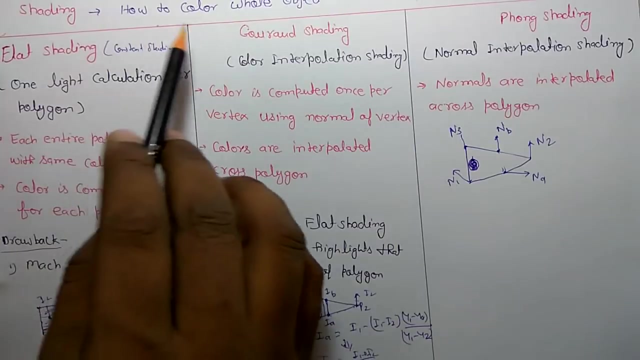 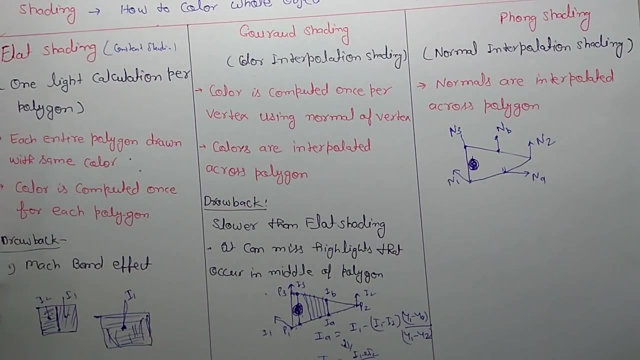 and do coloring. so our specular part is easily visible in fong setting. in fong setting you calculate normals at each pixel. that is why it is slower than gorar setting. so shading is the method. how can you color whole object? and in fong setting? here also you can use interpolation method. 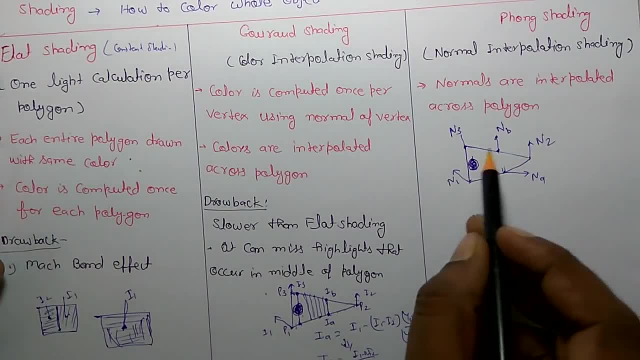 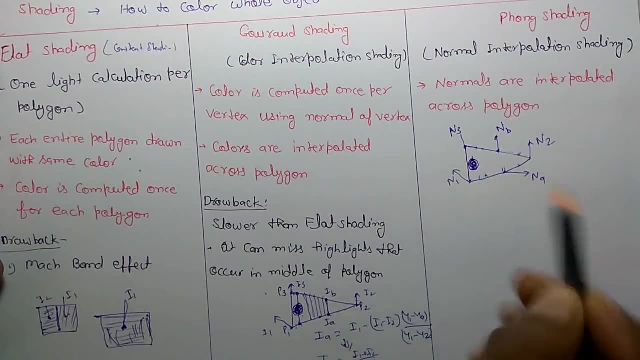 like here, we have used linear interpolation method. similarly, by using interpolation method, you can calculate normal vector at different pixel and find its intensity, and after that you can perform coloring. thank you,